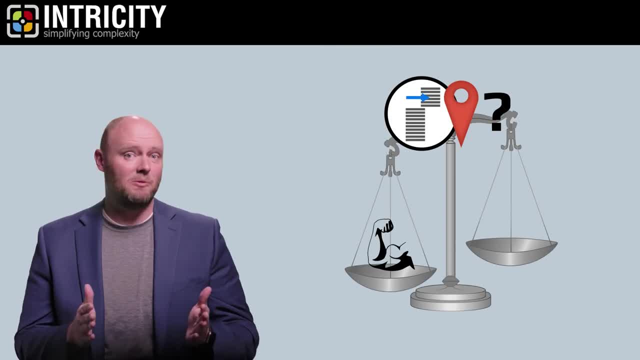 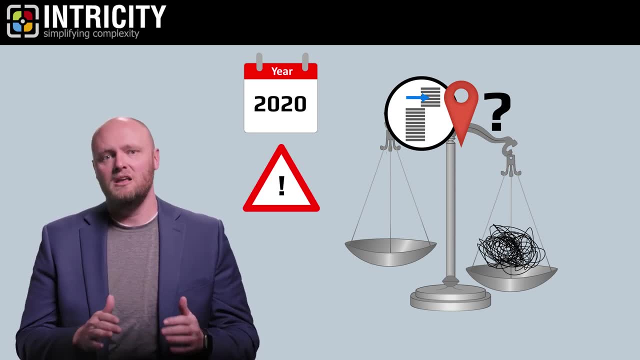 When it comes to access control, it can be the difference between enablement or total chaos. In recent years, access control has become a primary stumbling block in large data architectures. Now let me give you some contextual history to explain why. 20 years ago, we had a very complex data structure. 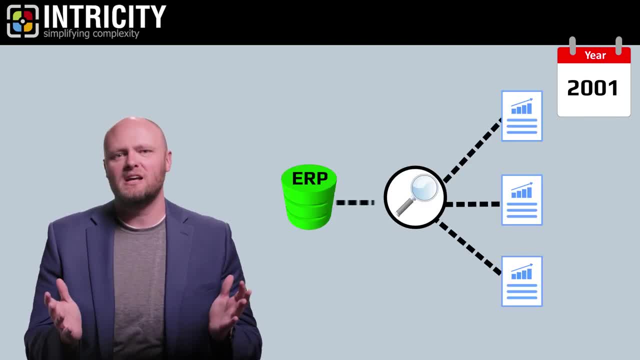 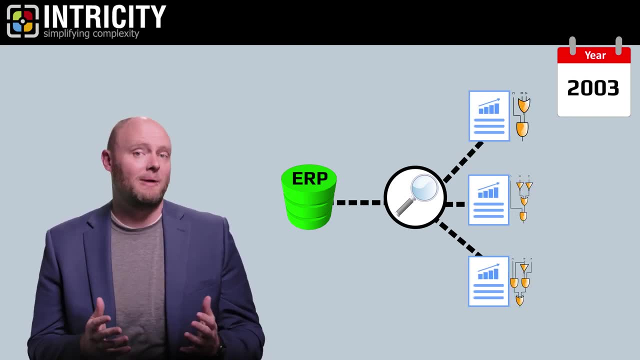 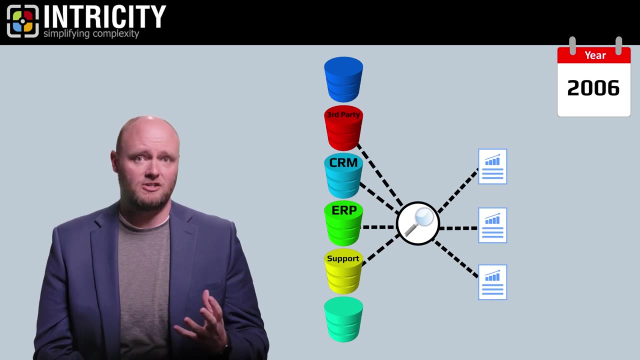 Data was mostly consumed through one-off business intelligence reporting applications. These systems housed all the complex queries for producing formatted reports. However, organizations began to see that the data itself needed more centralized logic. This was the time where wider adoption of data warehousing came into the picture. Access control still mostly lived in the business intelligence layer, even though the data had been somewhat centralized in a warehouse. In those early years, any consumption of the data outside of the data warehouse and BI layer was often considered as a rogue query. But this all began to change around 2015.. 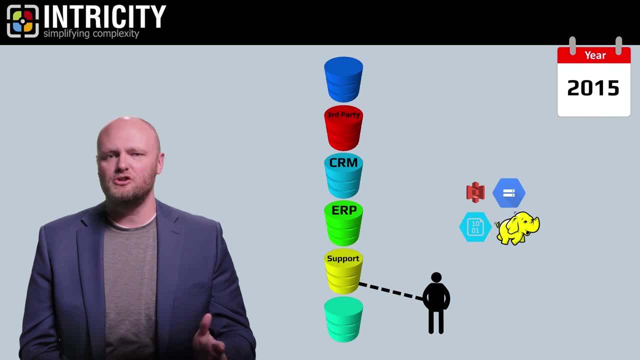 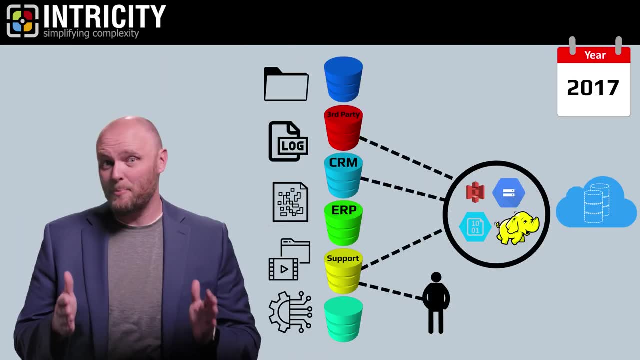 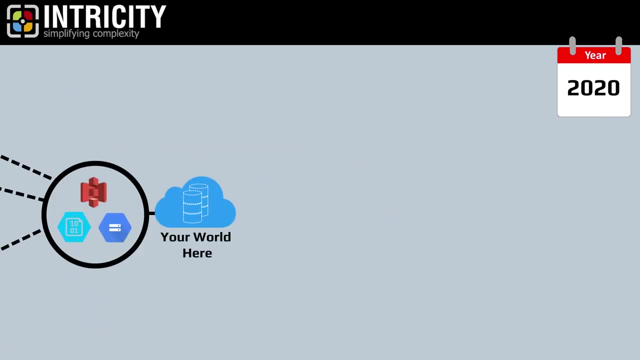 This is because cheap storage methods ushered in a centralization of data In more recent years. cloud data platforms have now made it possible to scalably query these deeply centralized data sets. With all this centralization, organizations need their data to be flexible. 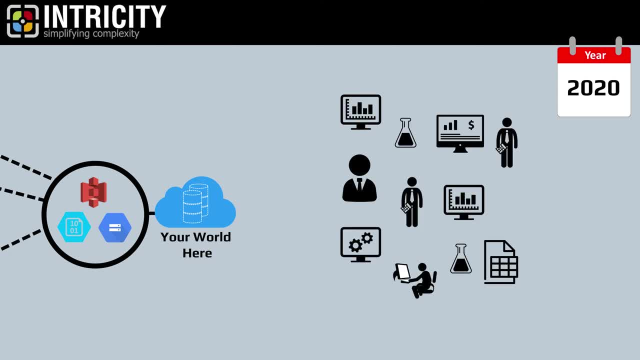 to an ever-growing number of tools and audiences. This means they can't just tightly couple all the access control into some reports and dashboards and then call it a day. Large organizations may end up having 10 business intelligence tools due to acquisitions and different end-user needs. 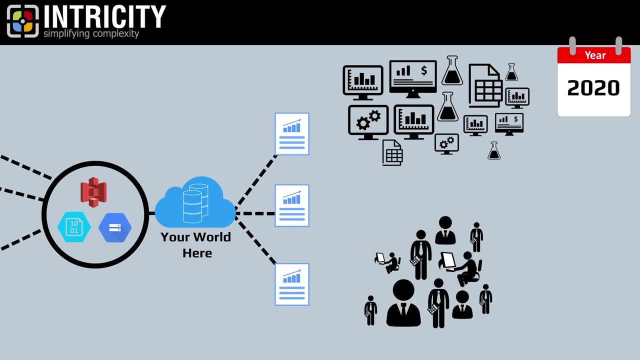 Additionally, they may have dozens of different audiences that interact with the data directly And not through some sanctioned analytics tool. So having access control nested into the BI layer no longer is a proposition that can suit today's large, modern data platforms. Instead, security needs to go back into the architecture. 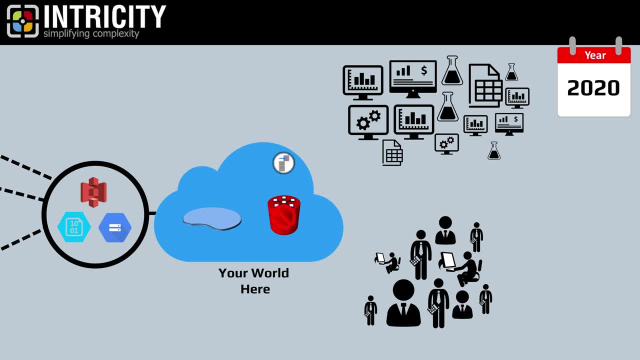 as an aspect of the data itself, And this doesn't mean the data warehouse, but rather even further back into the base data lake where all the core centralized data resides. This is the only way to ensure that any access control is able to be used in the data warehouse. 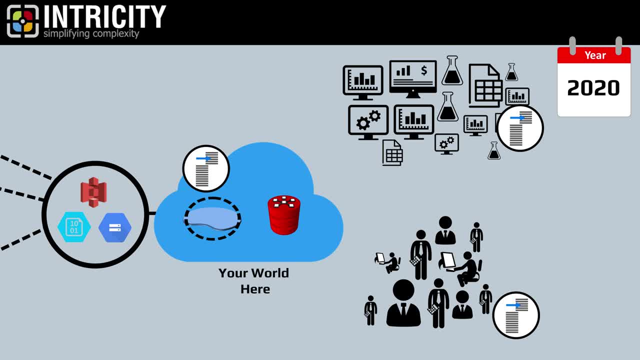 Access to the data can be segmented and relevant to the audience consuming it. Additionally, this makes it possible for any business intelligence, analytics, data science or reporting layer to plug into the environment and get consistent access based on credentials, and do so no matter if they queried the data warehouse.